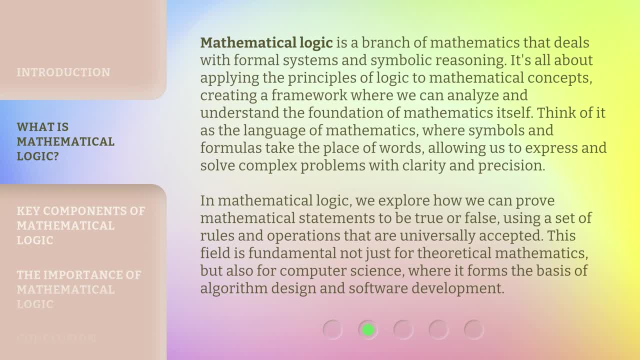 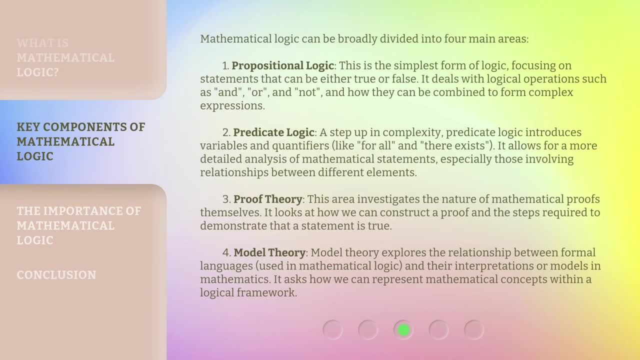 where it forms the basis of algorithm design and software development. Mathematical logic can be broadly divided into four main areas. 1. Propositional logic: This is the simplest form of logic, focusing on statements that can be either true or false. It deals with logical operations such as: 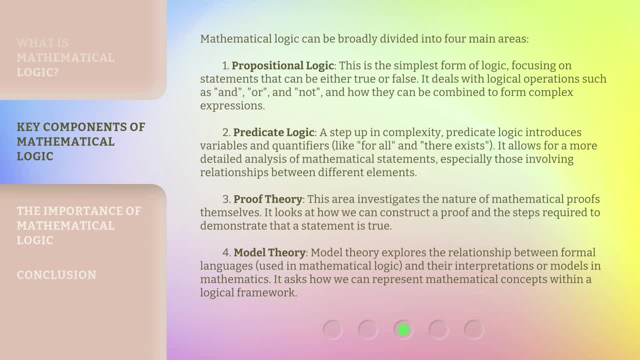 and or and not, and how they can be combined to form complex expressions. 2. Predicate logic: A step up in complexity. predicate logic introduces variables and quantifiers, like for all, and there exists. It allows for a more detailed analysis of 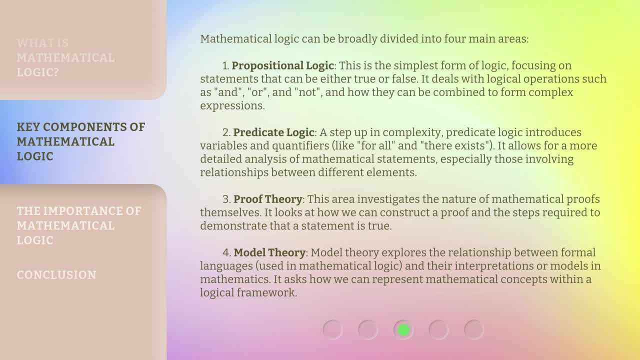 mathematical statements, especially those involving relationships between different elements. 3. Mathematical logic: This is the simplest form of mathematical statements, especially those involving relationships between different elements. 3. Proof theory: This area investigates the nature of mathematical proofs themselves. It looks at how we can construct a proof and the steps required to demonstrate that a statement is. 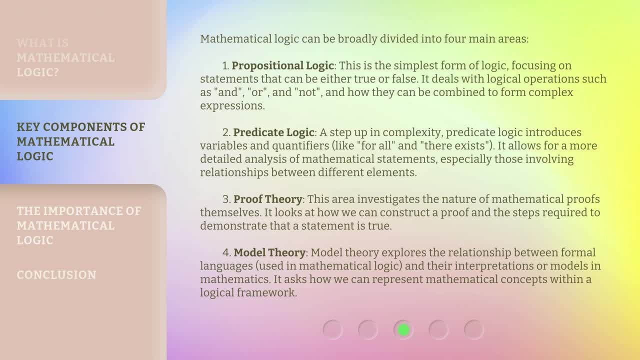 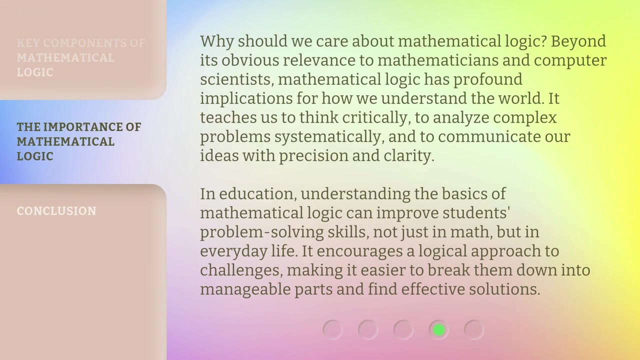 true. 4. Model theory. Model theory explores the relationship between formal languages used in mathematical logic and their interpretations or models in mathematics. It asks how we can represent mathematical concepts within a logical framework. 5. Why should we care about mathematical logic? 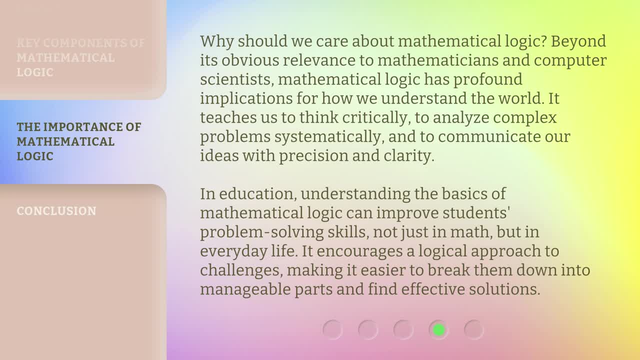 Beyond its obvious relevance to mathematicians and computer scientists, mathematical logic has profound implications for how we understand the world. It teaches us to think critically, to analyze complex problems systematically and to communicate our ideas with precision and clarity. In education, understanding the basics of 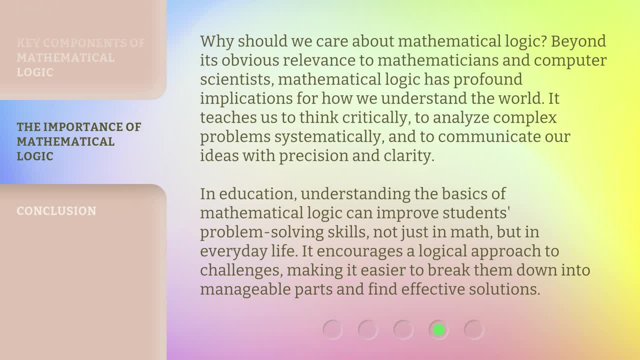 mathematical logic is a key part of our lives. It teaches us to think critically, to analyze complex problems systematically and to communicate our ideas with precision and clarity. Mathematical logic can improve students' problem-solving skills, not just in math but in everyday life. It encourages a logical approach to challenges. 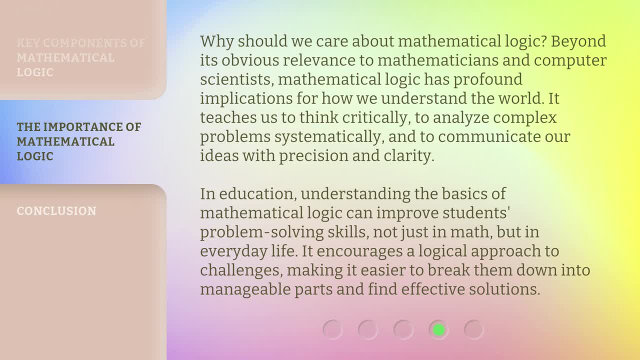 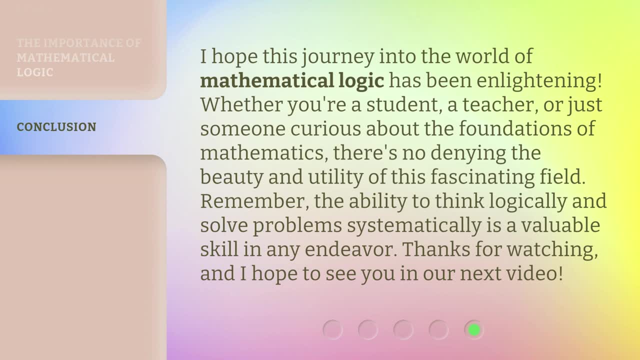 making it easier to break them down into manageable parts and find effective solutions. I hope this journey into the world of mathematical logic has been enlightening. Whether you're a student, a teacher or just someone curious about the foundations of mathematics, there's no denying the beauty and utility of this fascinating field.